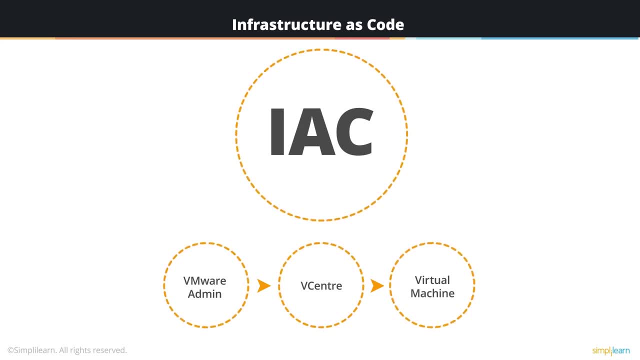 could not scale to a modern implementation that involves managing hundreds of VMs. This led to the development of Infrastructure as Code or Programmable Infrastructure and is the way that most companies today provision their infrastructure, whether it be virtual machines or containers. IAC is at the heart of current DevOps implementation and allows for the provisioning management. 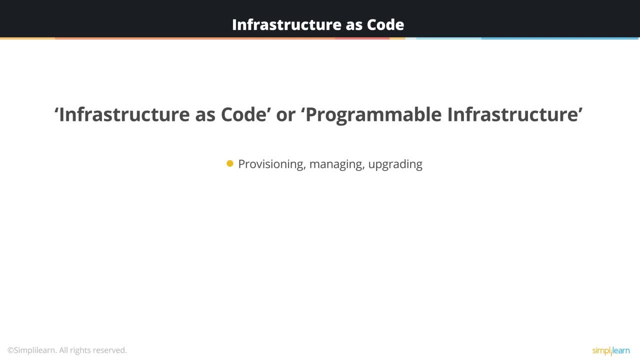 and update of infrastructure. Each of the configuration management tools have domain specific language, for example, Puppet, Chef and Terraform. Since these tools and their output in effect represent the working states of our infrastructure, it allows us to view and treat our infrastructure as if it's code, for example in the design. 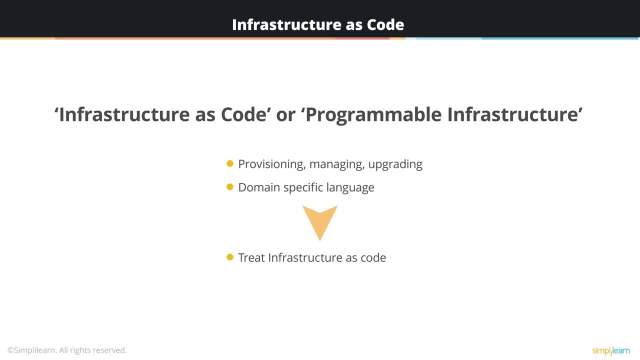 and release cycles and maintenance and versioning. IAC Features and Advantages. So then, what are the features and benefits of treating our infrastructure as code? IAC Features and Advantages. The first is code. The first advantage is that it makes our infrastructure versionable. 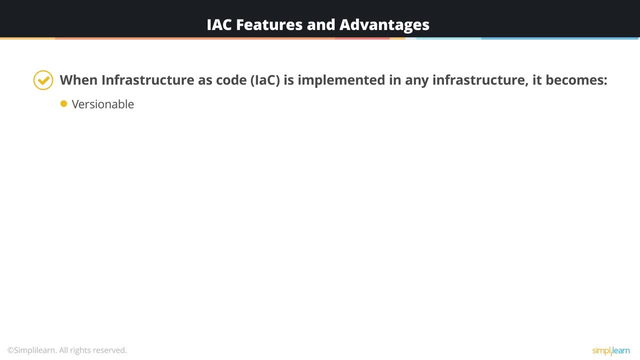 For instance, perhaps we need to roll back our infrastructure to a previous state due to a loading issue. Since the infrastructure is maintained in our VCS system, we simply select the relevant release by date or version and deploy that configuration. We can also use the VCS system to see the result of incremental changes to infrastructure. 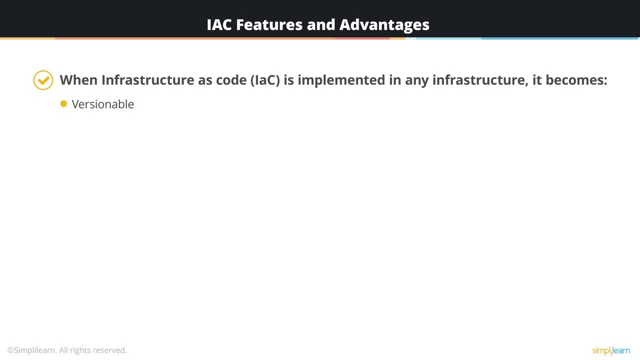 over time. This can be a powerful way to diagnose problems. The configuration is testable, Just as we test other software before we deploy it. our infrastructure code may be sandboxed and tested before deployment. It's repeatable. Since the infrastructure is implemented as code, we can efficiently replicate any infrastructure. 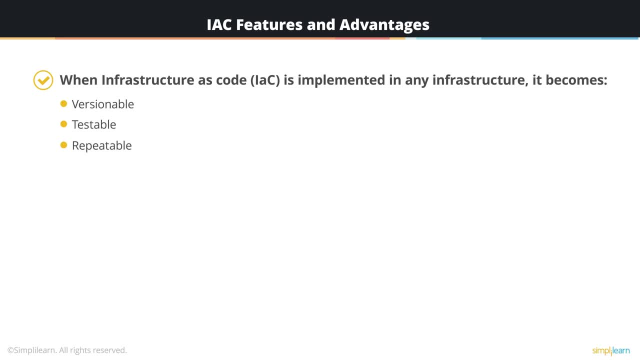 element in an accurate and scalable way. Whether it is one or a thousand elements, they will all be deployed identically. Additionally, this allows for parallel deployment. For instance, if we want to deploy a single infrastructure element, we can use the VCS. 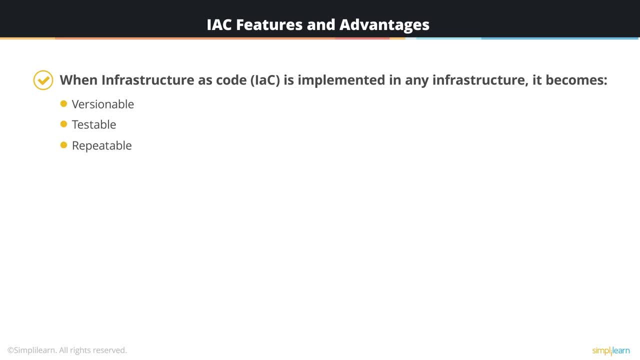 system. For instance, if one element of infrastructure takes 15 minutes to deploy, a thousand would take over 250 hours. However, since we have implemented our infrastructure as code, we may take advantage of multiple physical resources, so that our provisioning time will be the same. 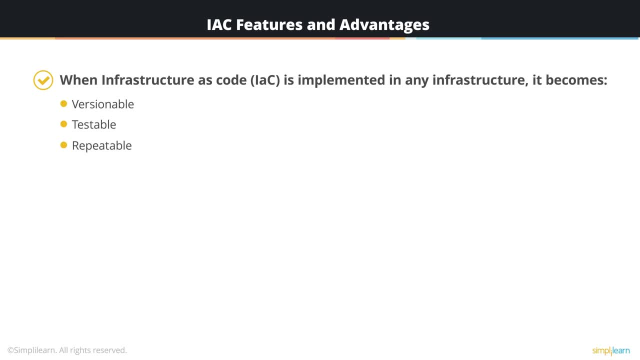 regardless of scale. This is one of the most important features of IAC. Popular IAC Tools Chef: This is one of the most popular tools for infrastructure as code and configuration management. Puppet- The biggest competitor of Chef is Puppet. Puppet was actually in the marketplace earlier than Chef, but these two offerings comprise: 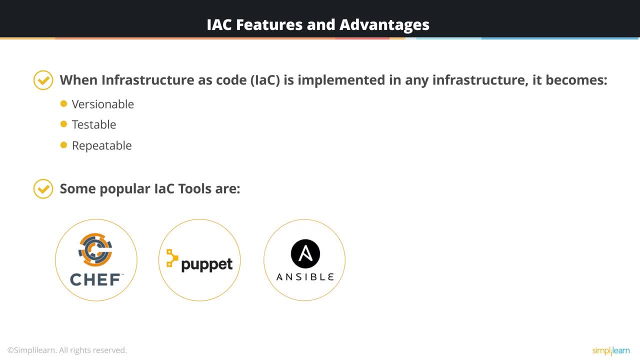 the largest share of the market Ansible. This is actually owned by Red Hat. It is a comparatively new product but has gained immense popularity in the last couple of months and is, in fact, almost as popular as Chef and Puppet and is gaining in market. 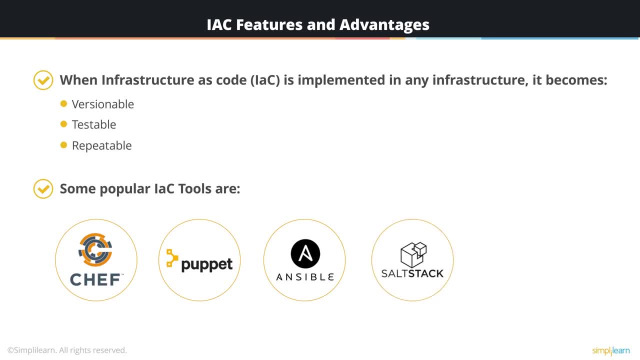 share. SaltStack Has many robust features and many companies have standardized on it. Also worth mentioning are PowerShell, DSC, CFEngine, BladeLogic and other various tools. However, the first four are probably the most widely adopted infrastructure and configuration management tools at this time. 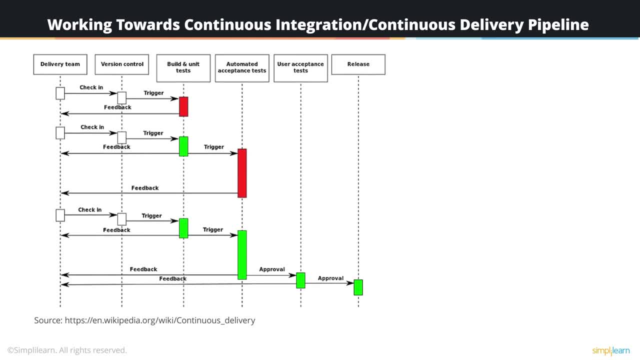 Working Towards CI-CD Pipeline, CICD Pipeline, CICD Pipeline. The current DevOps methodology is to be constantly working towards a CI-CD pipeline, where CI-CD stands for Continuous Integration, Continuous Delivery. This principle is central to DevOps. 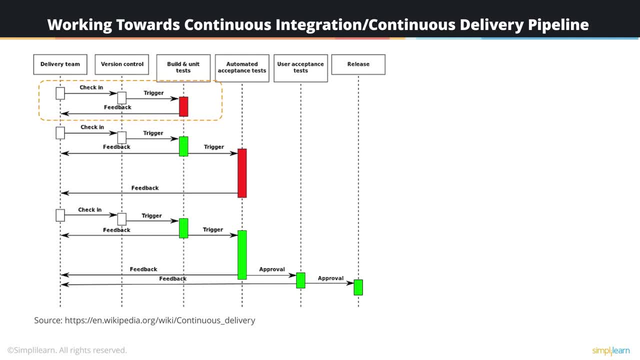 The goal is to achieve a pipeline where development changes move from phase to phase in a seamless manner through a series of triggers and feedback loops. Each phase is continuous with feedback until the trigger conditions are met. Only then, Once all contingencies are met, can the next phase be initiated. 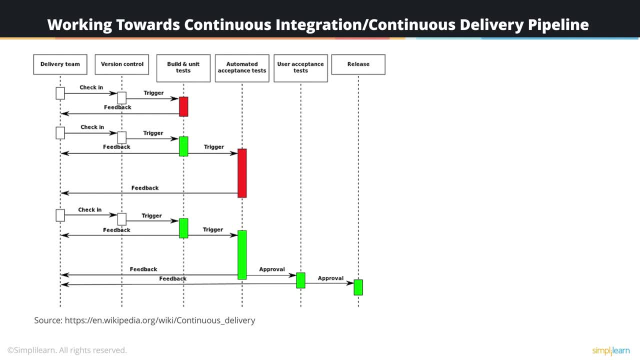 Additionally, each stage is automated such that, for instance, when a change is entered into the VCS system, this either initiates a feedback condition or automatically triggers a build and test cycle. There are various automation tools available to implement a CI pipeline. 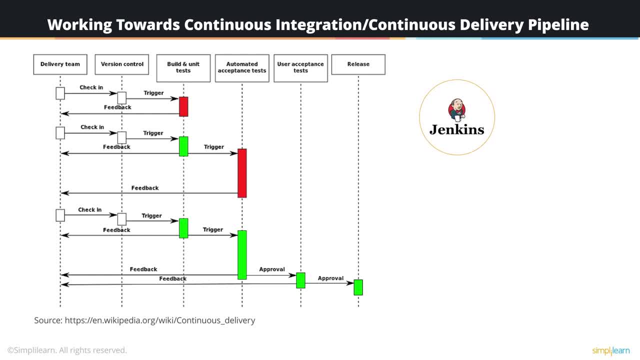 The most popular by far is Jenkins, but others like Bamboo, TeamCity and CircleCI are common as well. Each trigger point can be automated such that we have automated builds, automated testing, automated deployments, automated provisioning, etc. The key point here is to implement a pipeline that is integrated, seamless and error-free. 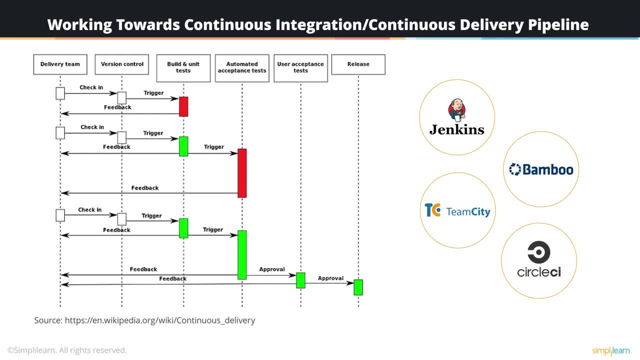 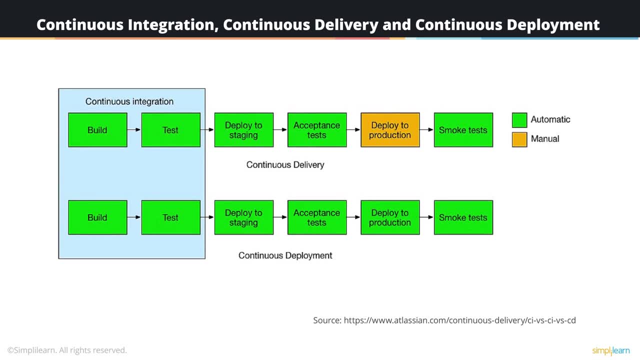 So then, the entire cycle from the developer writing code to deployment is known as the CI-CD pipeline. Three buzzwords for CI-CD that we will hear are Continuous Integration, Continuous Delivery and Continuous Deployment. There is a small but significant difference between Continuous Delivery and Continuous. 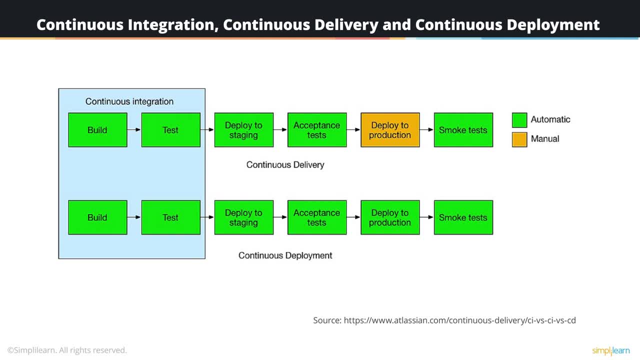 Deployment, which we will want to highlight here. The Continuous Integration phase is the same for both Continuous Delivery and Continuous Deployment. In both models, the developers commit their changes and this initiates a build and test cycle that ultimately triggers the next phase in the pipeline. 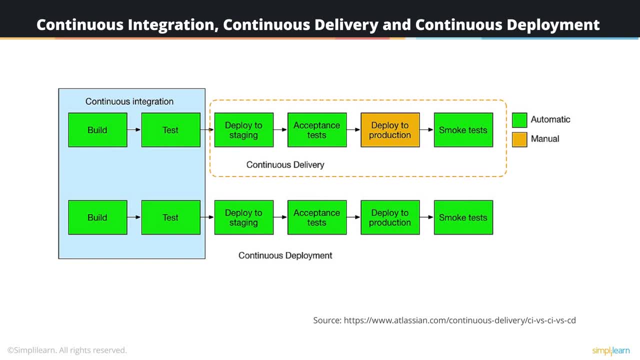 However, if you look at the top pipeline labeled Continuous Delivery, the deployment is the deploy to production box is orange. This is to point out the fact that the Continuous Delivery model follows the prearranged release cycle of the software. In other words, the changes are pushed out manually when the next software release occurs. 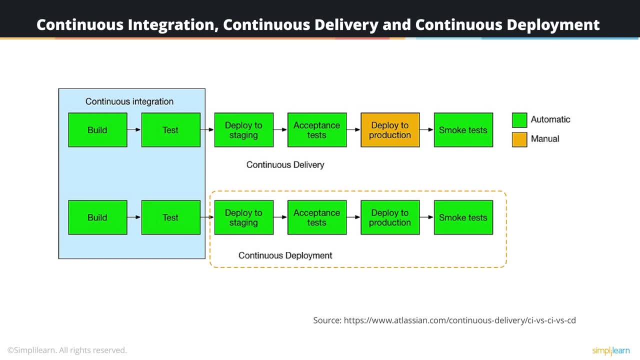 for example, annually. With Continuous Deployment, the changes are pushed out automatically as soon as they trigger the smoke test phase. This Continuous Deployment model makes changes available immediately throughout the pipeline. In other words, the changes are pushed out automatically as soon as the next software release. 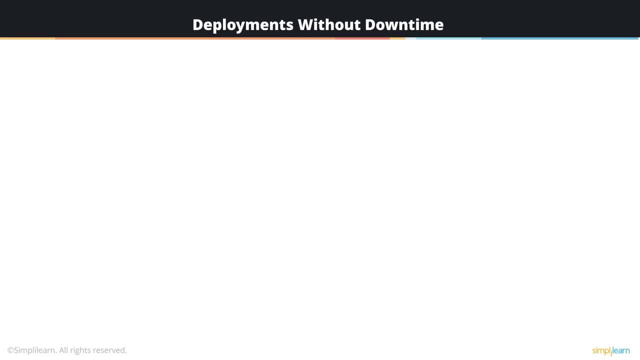 cycle occurs: Deployments and Downtime. Another key feature of modern DevOps is the ability to deploy without downtime. There are a few different deployment strategies that we can follow to minimize downtime. They are: Rolling Updates, Blue-Green Deployments, Canary Deployments. 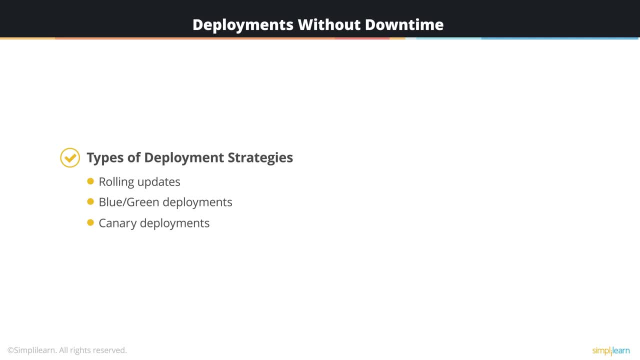 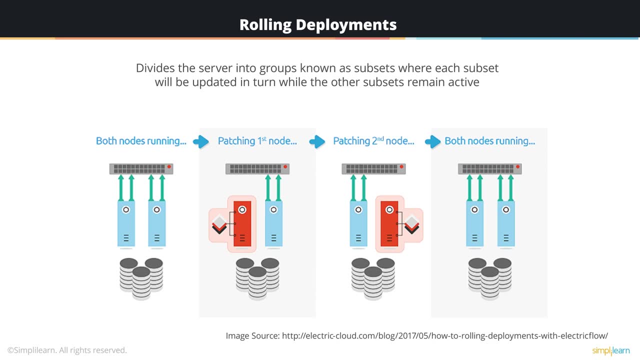 Let's look at each one to see how they compare Rolling Deployments. Rolling Deployments divides the server form into groups known as subsets, where each subset will be updated in turn, while the other subsets remain active. So, for example, if we had 100 servers, we might make 4 subsets of 25 servers apiece. 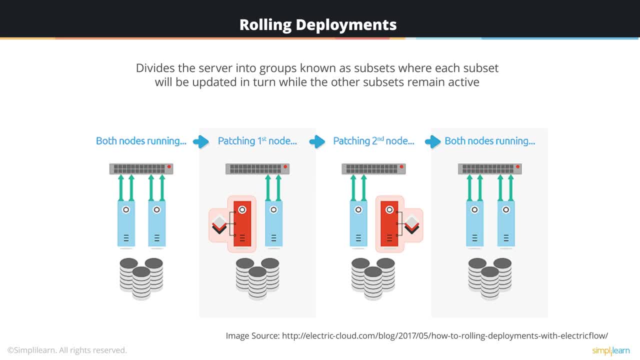 Now we can batch update the first subset of 25, while the remaining 75 servers are still actively serving the application to end users. Now we can restart the first subset and continue the process with the next subset and still maintain 75 servers active through the entire deployment. 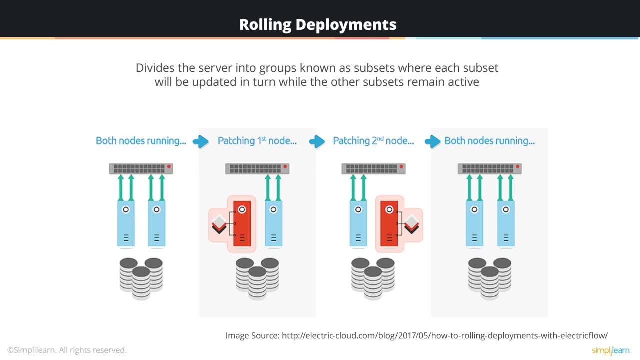 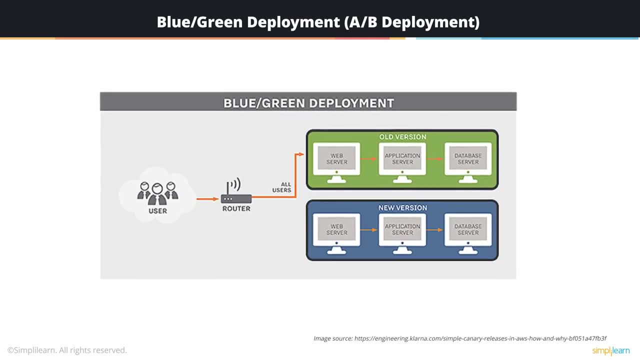 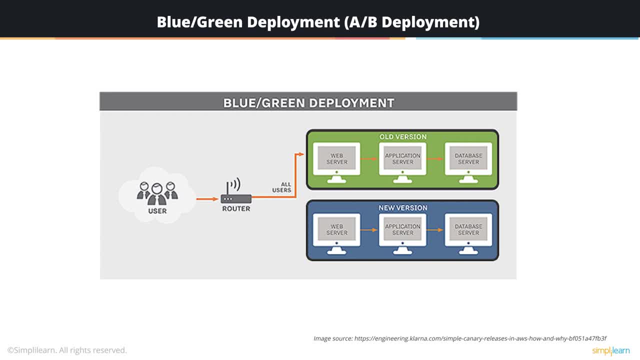 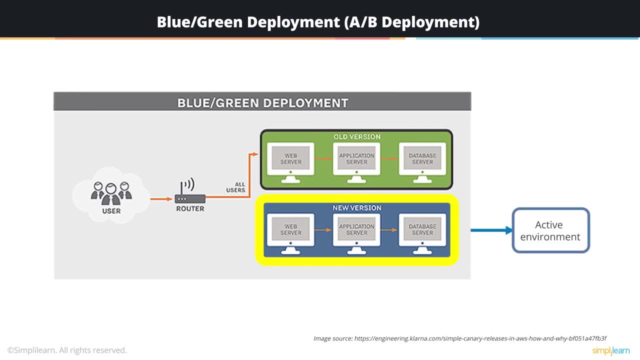 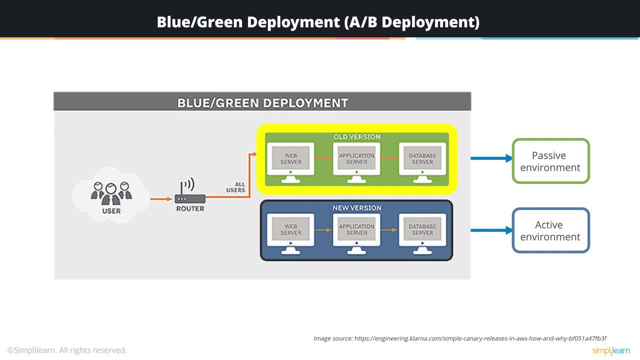 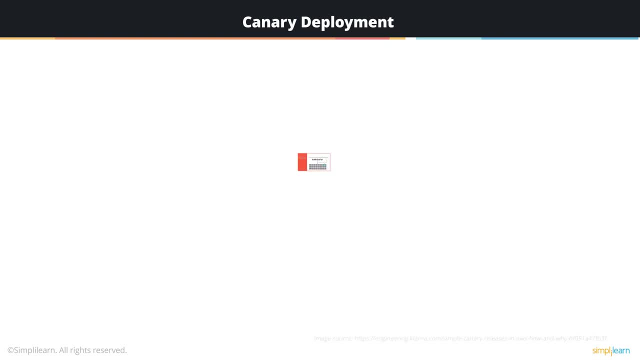 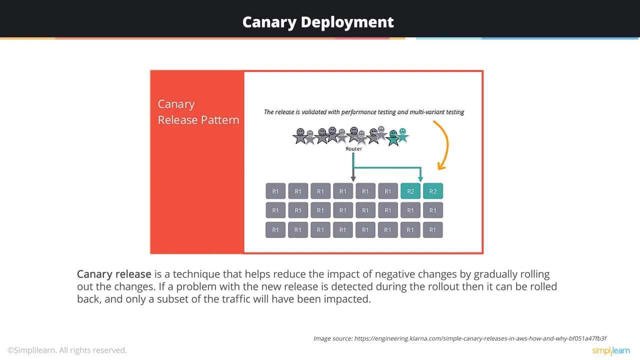 Then at some point the passive environment is activated and the user base is served from the updated environment. The third method of deployment is known as Canary Deployment. This methodology has become extremely popular recently and is used by giants like Amazon and Netflix, With Canary development only a small subset of servers. 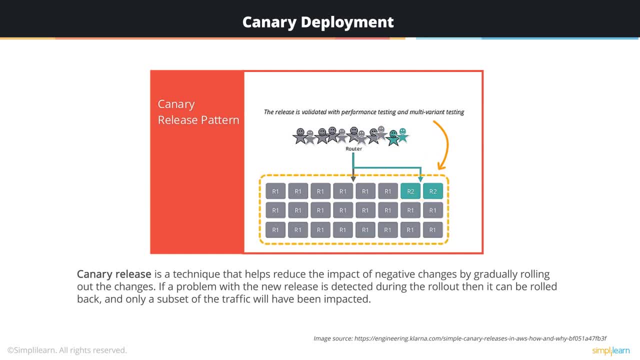 is updated with the changes. If the changes cause no problems, the changes are rolled out further and monitored again. This cycle continues until the entire user base is included. At any time in the process, if problems are identified, the updates can be rolled back. This enables two. 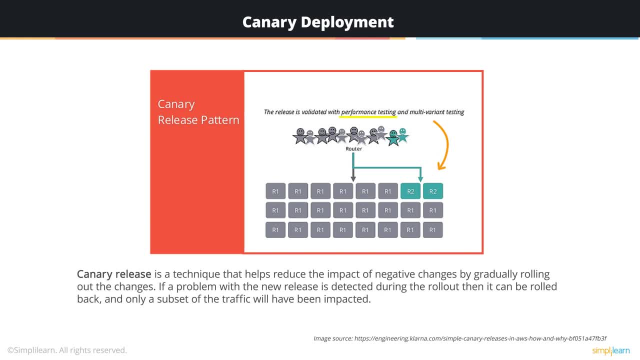 very powerful strategies. The first is performance and quality testing to a defined subset of users. The second use case is multivariant testing. Here there may be some uncertainty as to which feature set best serves a user base. The Canary method allows the software producer to test the 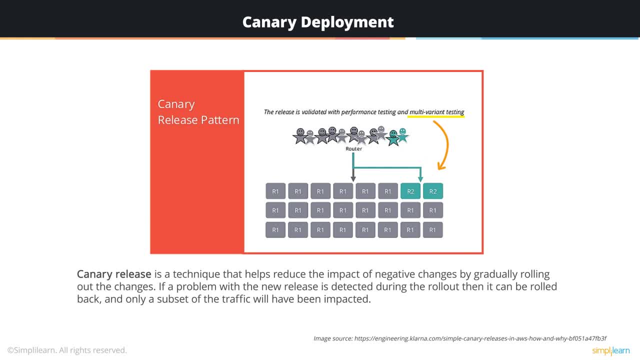 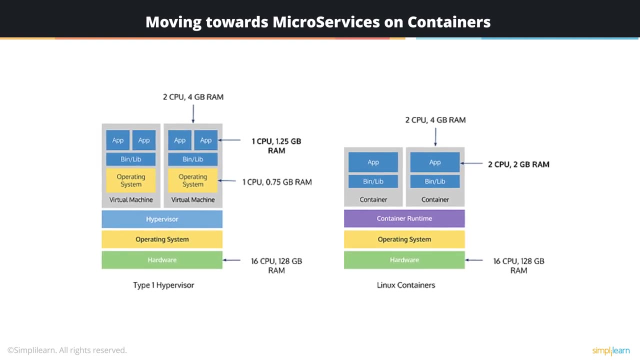 variant feature sets on defined subsets of the user group to determine acceptability. Once the determination is made, the final version can be deployed to all users. Moving towards microservices on containers: The next key to modern DevOps practice is the move towards microservices In traditional monolithic software development: a single virtual. 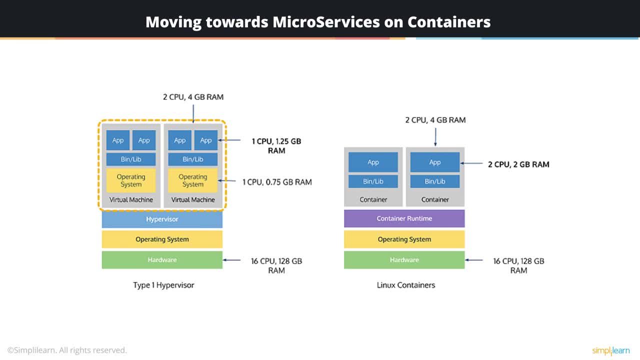 machine would be dedicated to serving an application. However, with the advent of microservices, using an entire virtual machine to deploy a microservice is costly from a resource as well as a performance standpoint. Companies today are using containers for their microservices deployments: Containers- 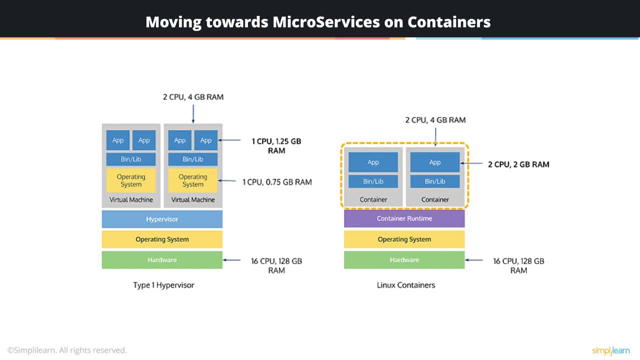 have completely changed the way we deploy, manage and maintain our applications. This is why all major cloud service providers, such as AWS, Azure and Google Cloud, have integrated Docker and provide containers as a service. Let's take a look at some of the benefits of containers. 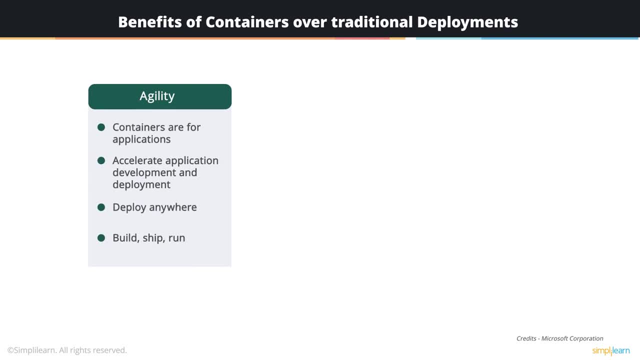 If you use containers in your software deployment, they will become more agile. By that we mean you can use containers to deploy applications. By compartmentalizing you can accelerate application development, test and deployment. Package dependencies means you can deploy anywhere. Containers suit the continuous deployment methodology and enable build, ship and run. 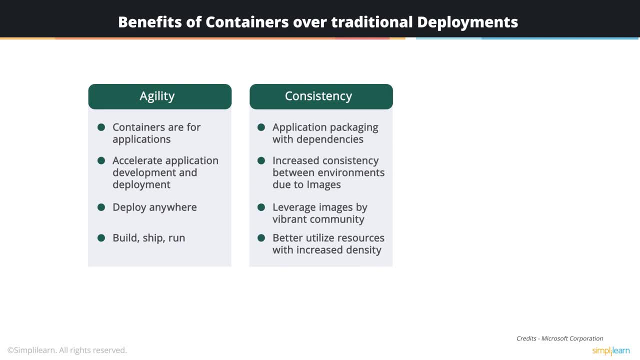 Consistency. Consistency is the key to successful releases In the monolithic deployment methodology. environmental inconsistencies are the main cause of failed deployments. Small differences between the dev and test and deployment environments become major roadblocks to a successful deployment. Containers remove this roadblock by packaging all dependencies. 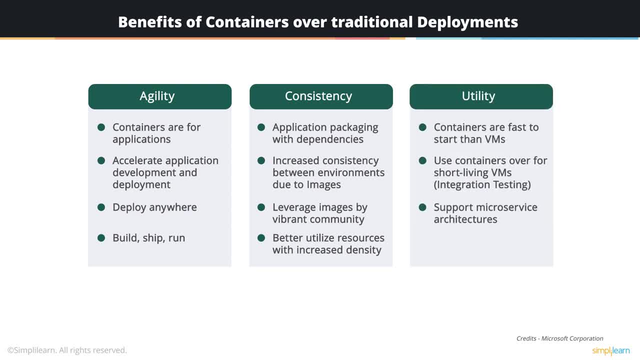 Utilities. Utilities: Containers start and run much more quickly than virtual machines: One second as opposed to one or two minutes or even more for a virtual machine. In particular, for small test cases, containers are ideal. Containers were designed to support the microservices architecture. 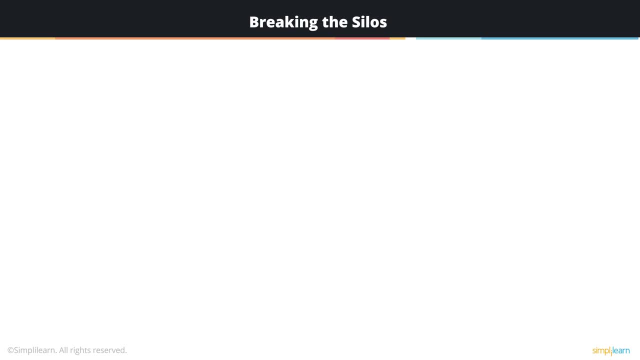 Breaking the silos. The final principle of DevOps is breaking the silos. When we talk about having an efficient CI-CD pipeline, we are presuming that we have collaboration. This means that developers, testers, operations personnel- anyone who is a business stakeholder- 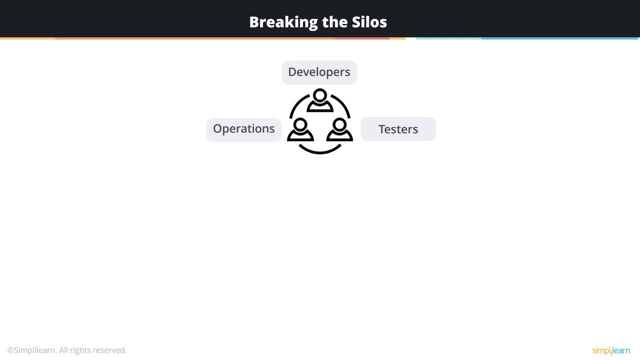 in your application should be working together. However, in large projects and large organizations, this is rarely the case. The traditional team structure, where teams are siloed by development operations, networking, storage, etc. is not the case, The traditional team structure. where teams are siloed by development operations, networking, storage, etc. is not the case. The traditional team structure where teams are siloed by development operations, networking, storage, etc. is not the case. The traditional team structure where teams are siloed by development.